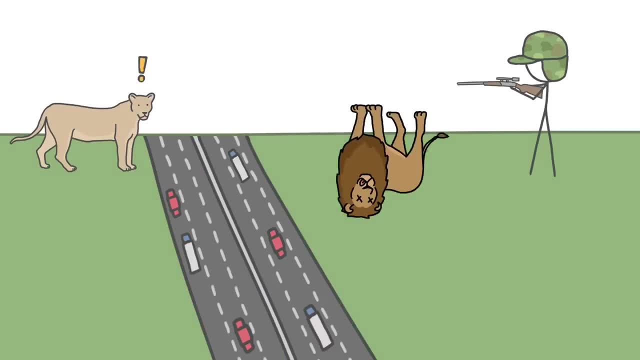 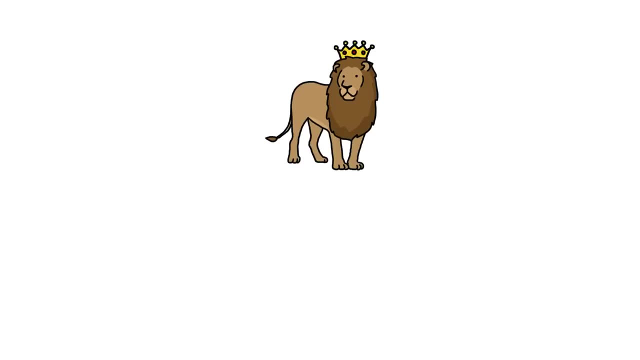 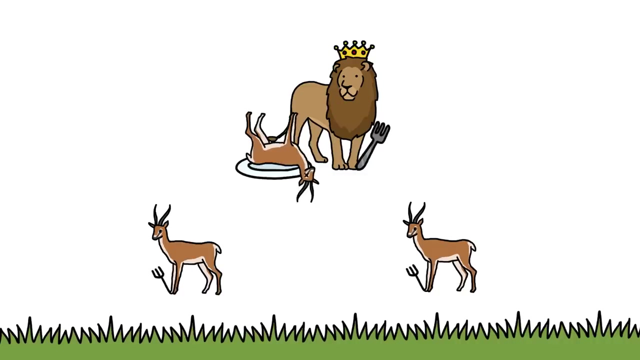 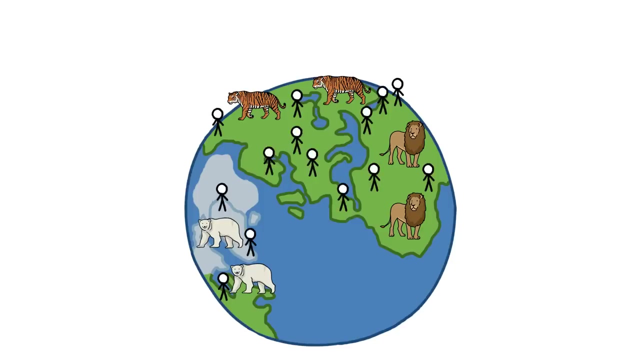 breaking up their habitats and hunting many of them to near extinction. We ate the plants and we ate their meat. Then this little ape called man wanted to compete, And as the humans spread and invaded globally, they broke up our habitats and killed us all. 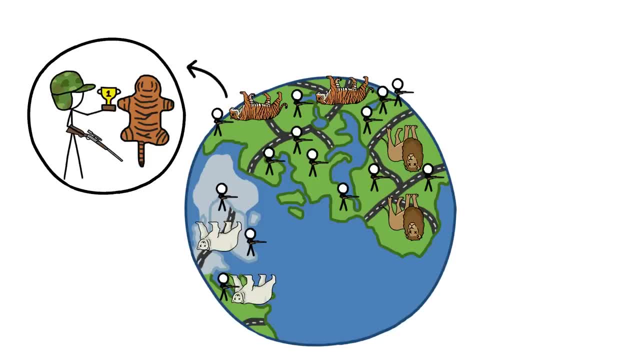 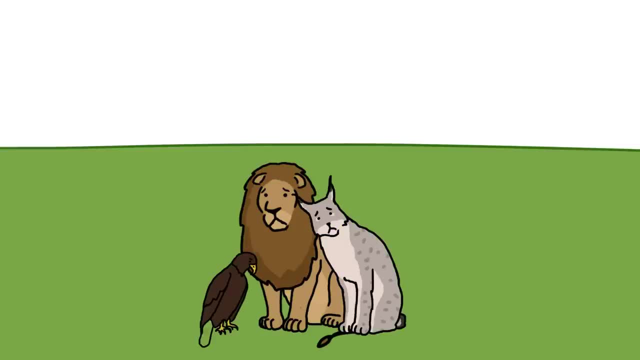 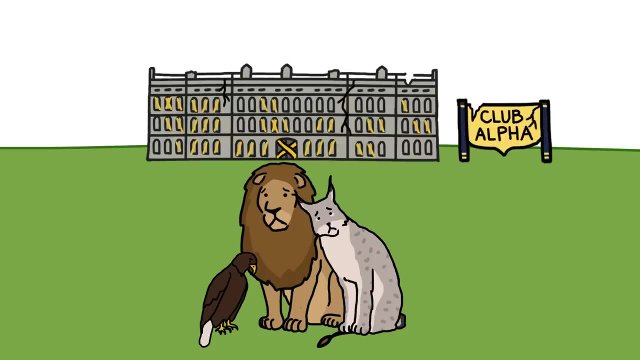 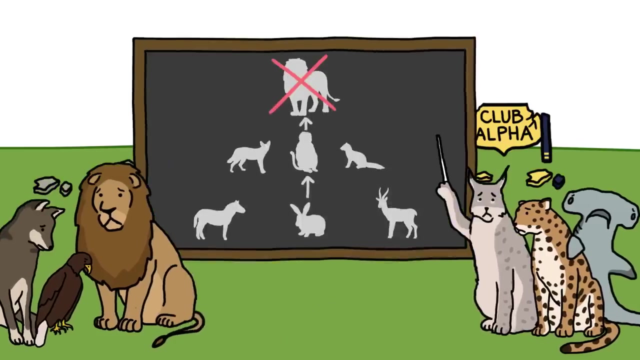 rather fast. They were shooting us for sports or eating sheep, Lions, lynx and seagulls- Alphas worldwide- met precipitous decline. Leopards, wolves and hammerheads were persecuted, leaving disarray behind. Not to throw shade, but this trophic downgrade will simply open up space for some lesser grade. 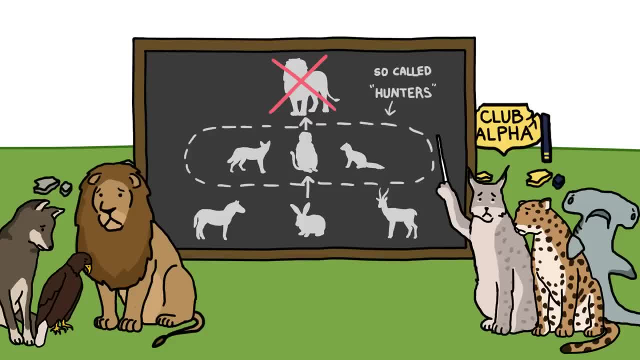 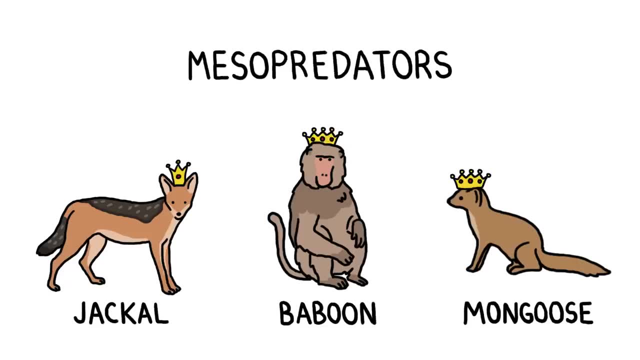 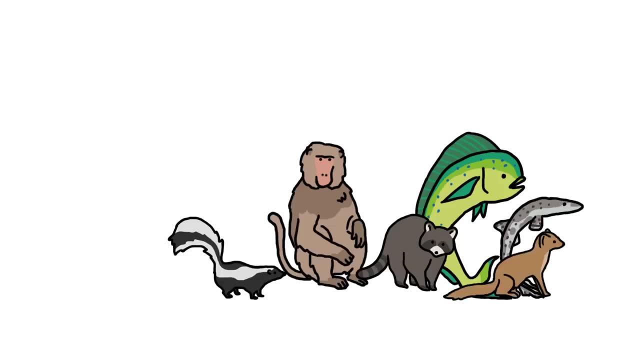 so-called apex predators. These so-called hunters are the mesopredators. They're replacing apex predators all over the world and they do things differently. Skunk raccoon, mahi-mahi, mongoose, cat shark, dogfish, jackal, large squid food chain. 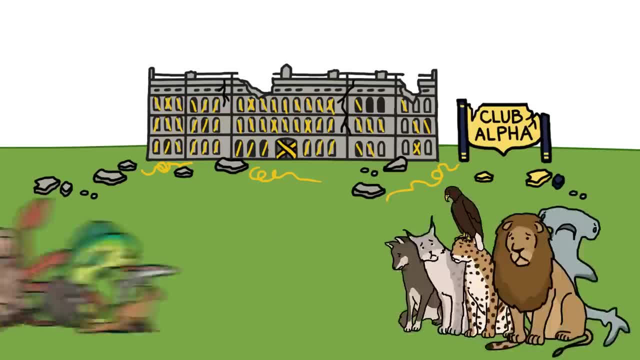 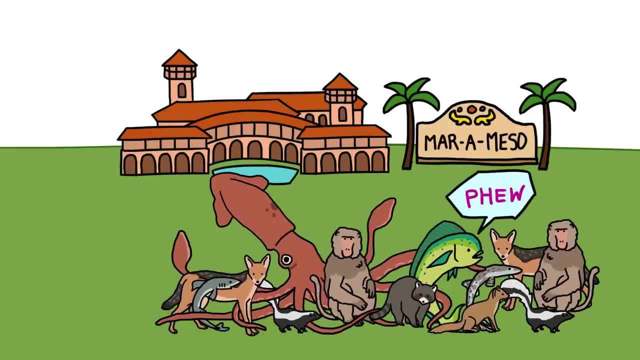 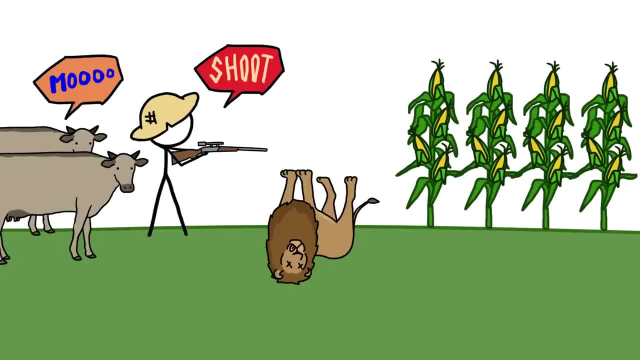 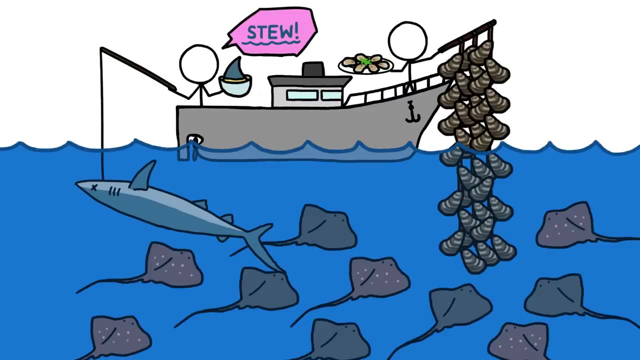 Say goodbye to our old foes. Yeah, what a relief. No competition or hunting. Mesopredators are released When farmers hunt down lions just to protect livestock. Nobody left to eat. baboons who start eating all the crops. Sharks getting killed for their fins. Boom time for the raisin skates. 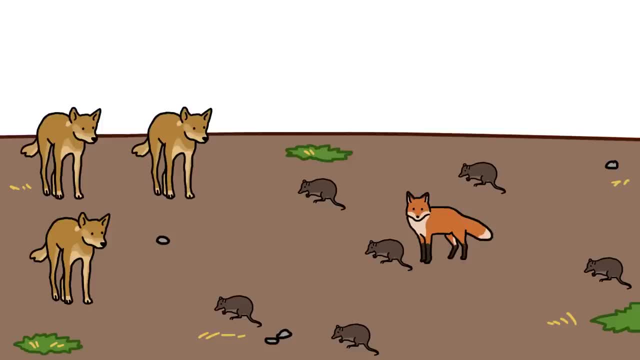 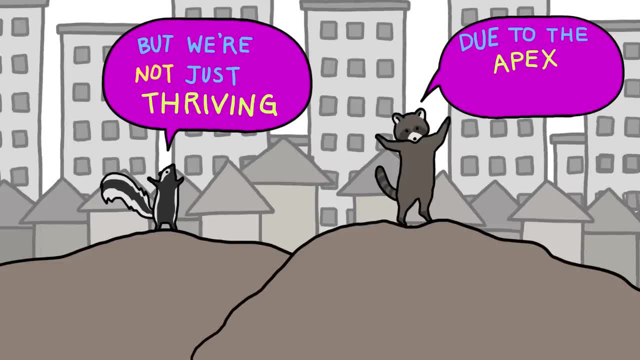